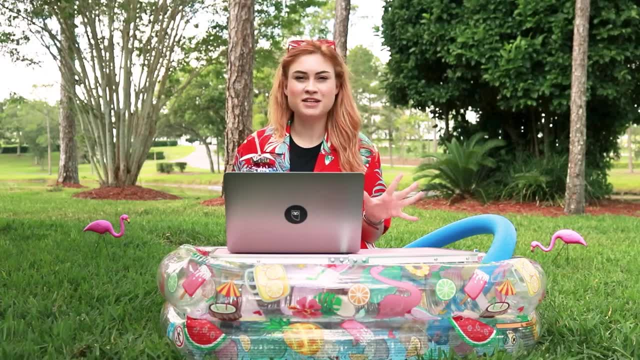 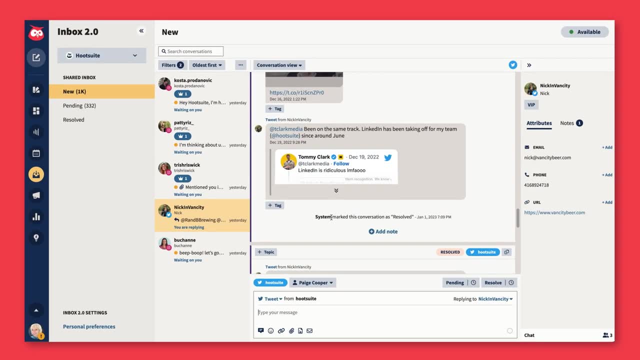 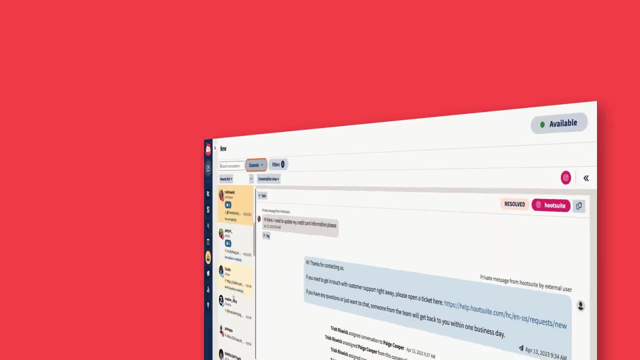 All your social media messages- private, public, dark, organic DMs, comments, emojis, mentions, questions. they are all in here in Hootsuite Inbox. Let me show you how Inbox bridges the gap between social media and customer service. So let's start with a conversation view which is: 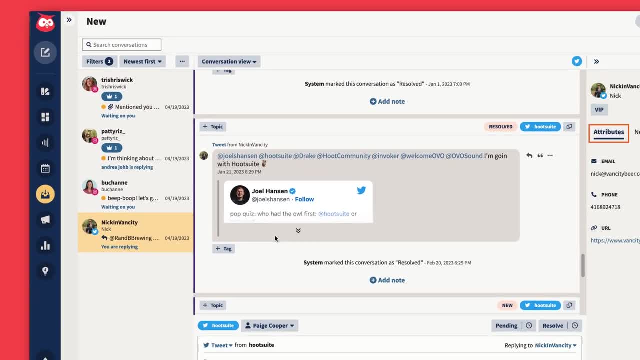 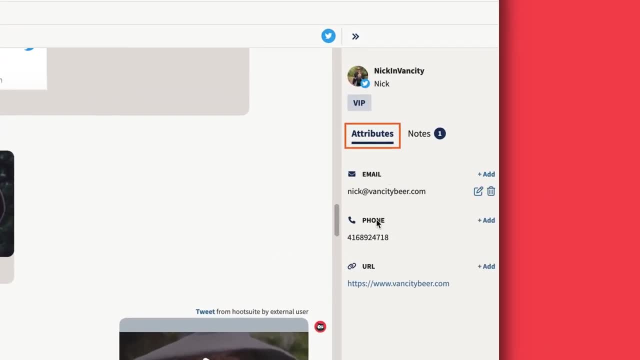 actually the entire history of a person's interaction with us. This honestly lets me be way more helpful than I would be if I had to start from scratch every time a person got in touch with us. If I go over to the right, I can see a customer's profile which has their contact. 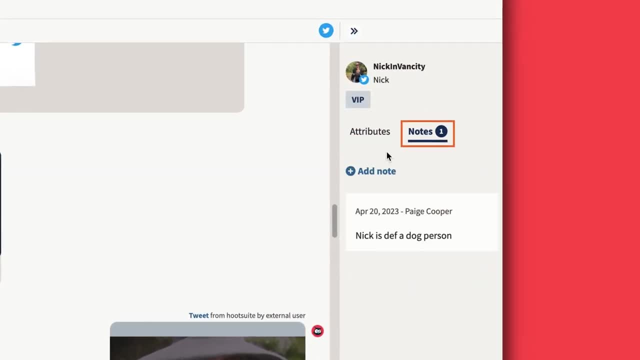 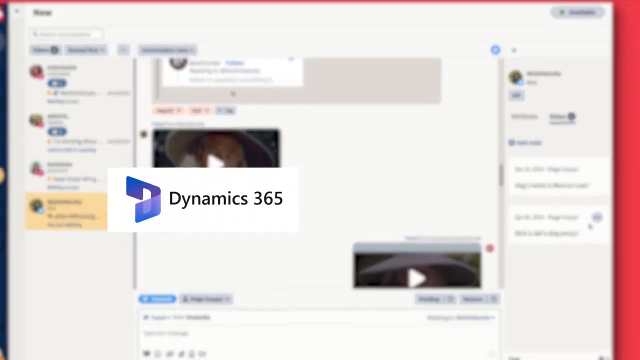 information pulled from our CRM and which I can edit and add to as I learn more about them. I like to check the notes in case there's something in here that helps me personalize my reply, And the cool thing is, anything I add in there also flows back to our CRM, so it helps our sales. 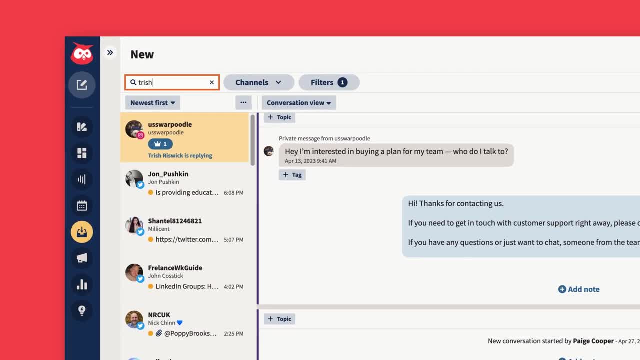 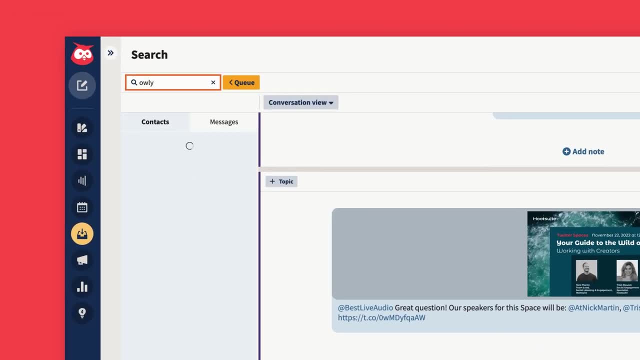 team too. Over here I can search all of our messages by keyword or customer, so I no longer need to memorize every conversation that we've ever had- Ever. A quick search is also a good way to take a pulse check to see if there's anything in here that I need to add. So let's start with. 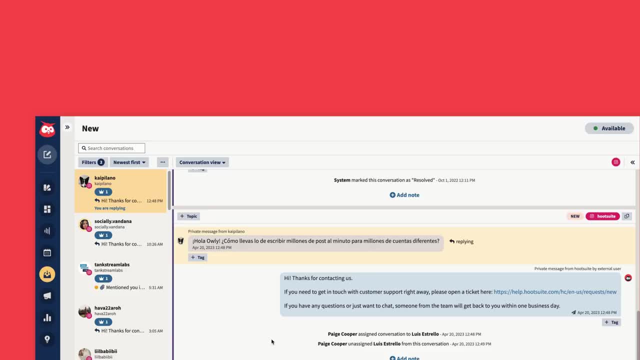 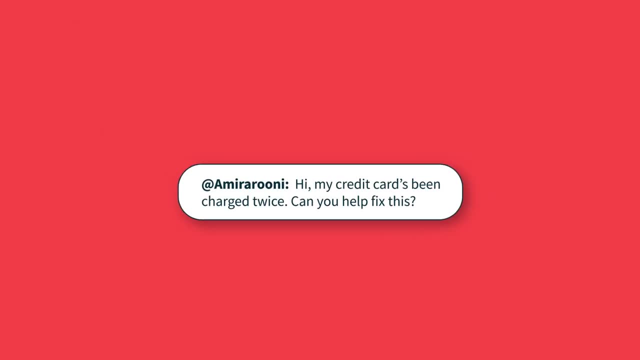 a certain topic, To assign the conversation to myself or to someone else. I just click here So I could search for Luis in customer support, who I know speaks Spanish. but I actually don't have to assign messages very often because Inbox automatically sends them to the right people. 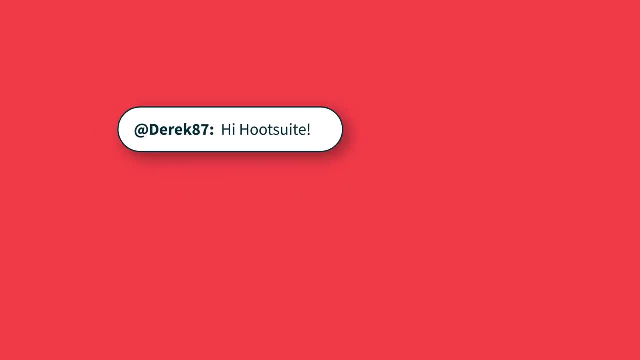 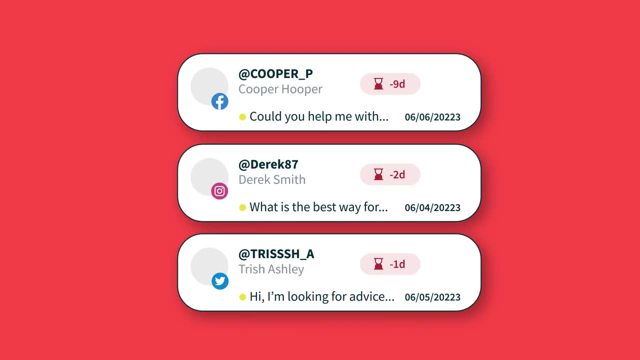 which cuts our response time down like crazy. You can automate other things too, like sending autoresponses, customer satisfaction surveys and SLA notifications, which is another huge time saver. And, of course, Inbox supports your chatbot technologically, end-to-monthly and online. So if you want to make sure that you're getting the most out of your 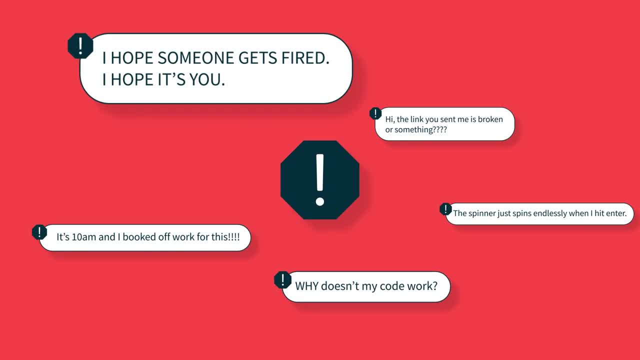 message. you can do that by clicking the link in the description below. Oh and one last thing. Last week Inbox flagged the mini-coms crisis so early that we were able to handle it using auto-replies and without escalating it to the big boss. It's priceless. 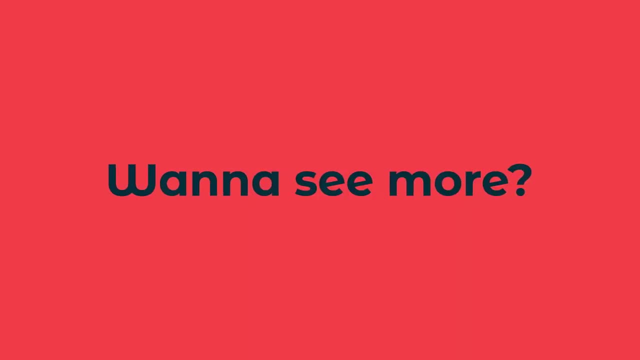 for our brand, safety and my mental health. Want to see more? Get in touch today.